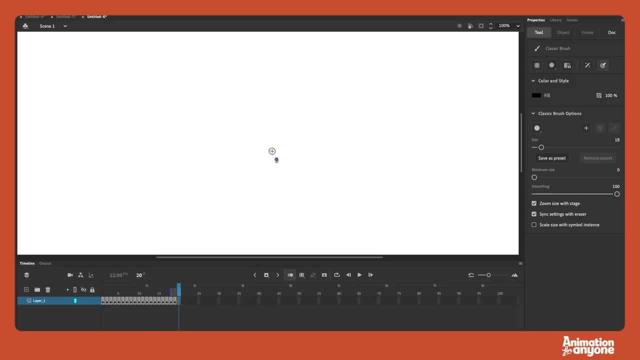 to do it. You can be a stop motion animator, you can be a motion graphics designer, you can be trying things out for the first time and you can really get a sense of what different spacing does to the speed and the energy of your motion. So if I want to make things move slowly, 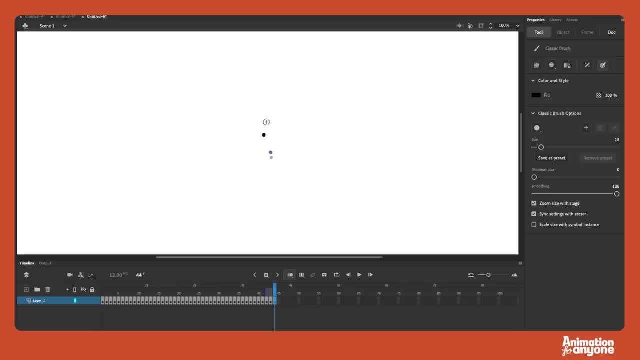 I make them close together and if I want to make them fast, I make them further apart. You can see I'm animating on arcs at the moment. Let's see what happens When I want to animate on a straight line, go nice and quick and slow down really quickly, and now maybe I want to do some extra fast motion. 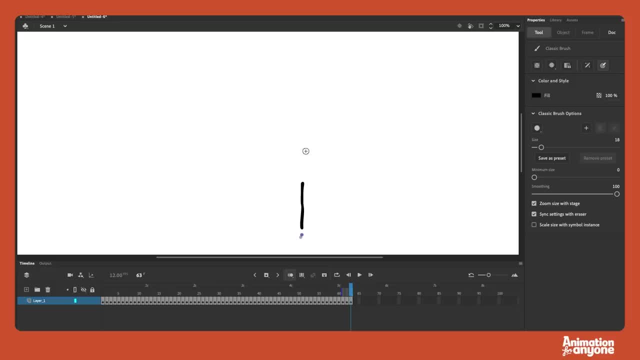 So I'm going to start using a smear. It's good to know that this isn't stretch or squash. this is a smear because it's using different volumes, So this is a bit more like a motion blur in live action footage. So I'm just going to smear this out. go really quick. 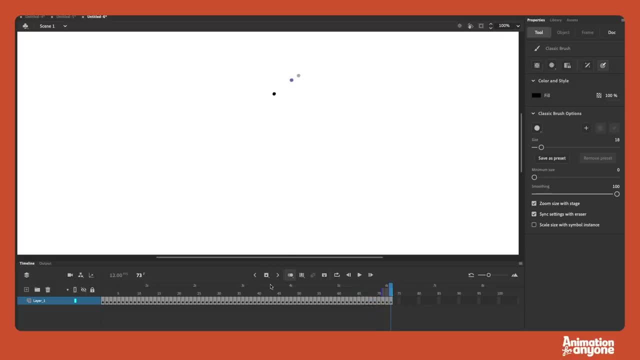 and then slow down really quickly. Let's see how that looks. Yeah, as you can see, you can get some really interesting movement very rapidly and you can just experiment, make mistakes, make new discoveries really quickly. This exercise is fast enough that you can do it multiple times and test out different ideas. 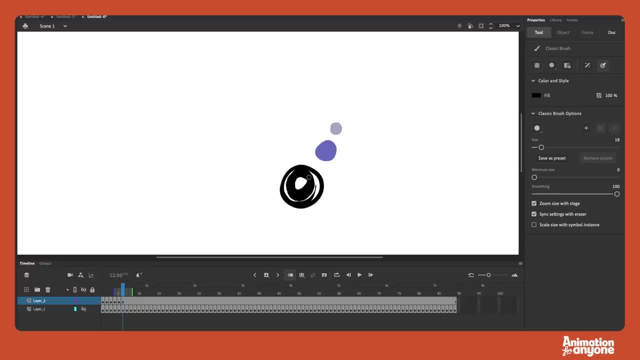 So I'm going to make a new layer on top of the old layer and try again. This time I'm going to try to add some depth to the image by making the dot bigger as it gets closer to us and smaller and have tighter spacing as it gets further away. 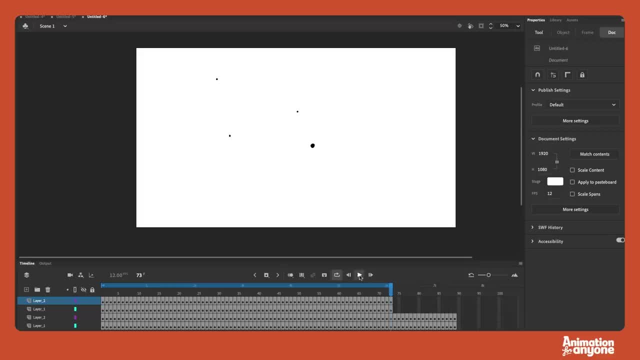 Each of these passes only takes, you know, a few minutes, so I'm able to play around with lots of little ideas. Just as an experiment, I decided to join all of these dots together and it created quite a cool abstract animation. It moves in a pretty appealing way and that's. 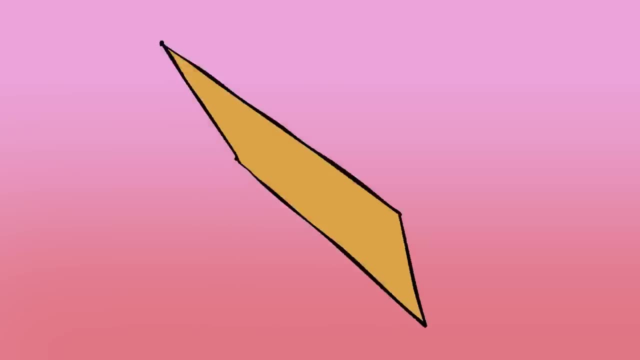 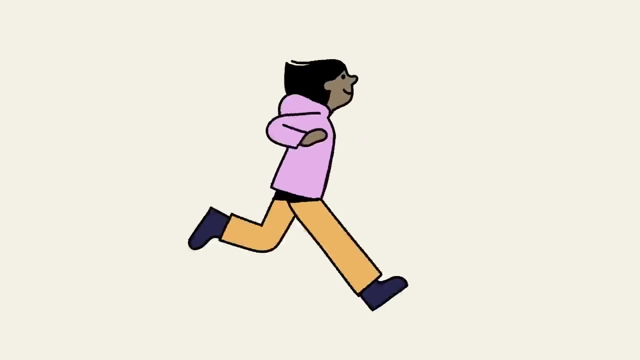 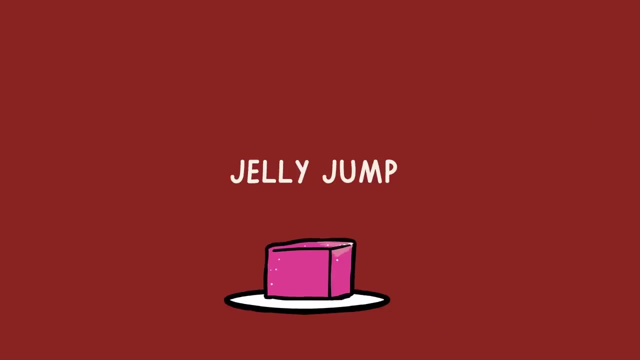 because all of the elements have special attention paid to their spacing and arcs. This won't just be the case for abstract animation. pretty much any object or character you animate will benefit from spacing and timing ideas that you learn with this exercise. Next up we have the jelly jump. In this exercise we're going to try to make a block of jelly. 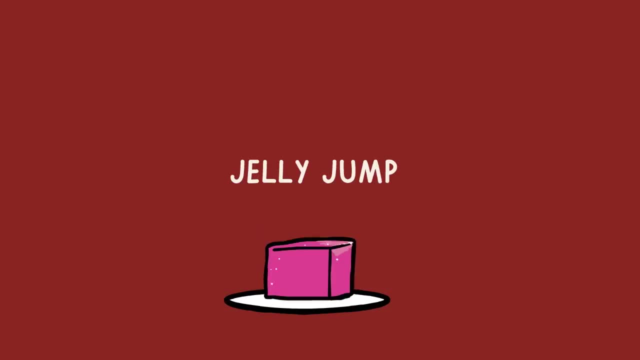 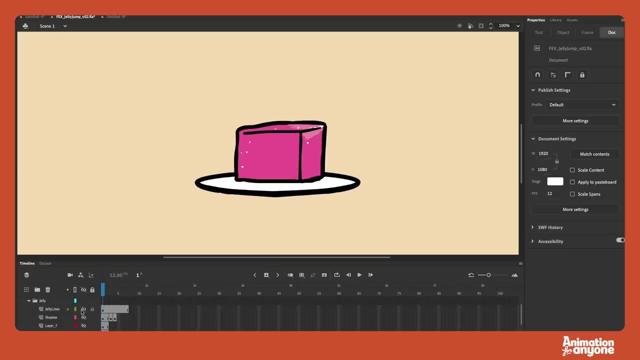 or jello, depending on where you live. jump in the air and settle down. We're focusing on creating weight using anticipation and overshoot. So we have a drawing of some jelly here in Animate CC. I've split it up into layers so that I can lock. 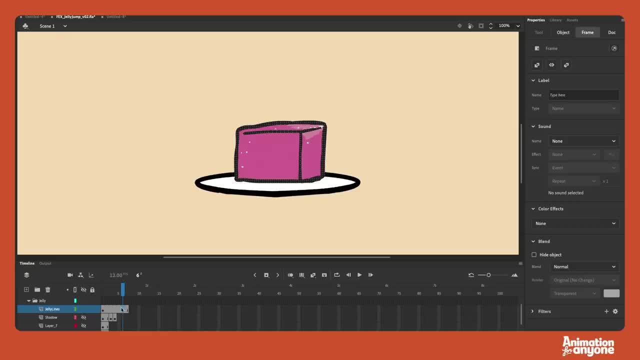 the background layers. The first thing I'm going to do is create the most important keyframes. So we've got our starting frame. I'll create a new frame at the top of the jump and I'll duplicate the first frame and use it as the final frame. I'll make it hold for a while by pressing F5 and I'll play that back. 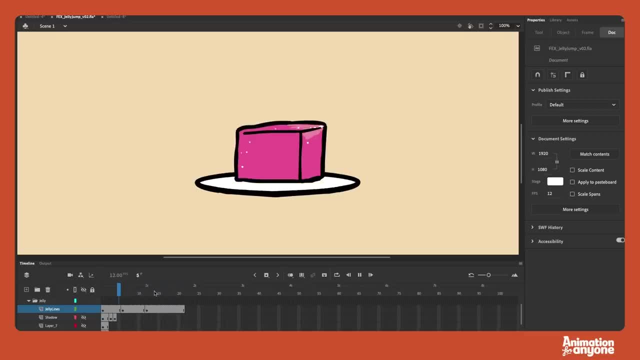 That doesn't really feel like a piece of jelly jumping right now. So what do I need to add? Well, I'm going to add an anticipation pose. So this is where it squishes down a little bit, and to do that rather than redrawing it, you can redraw it if you're so inclined. 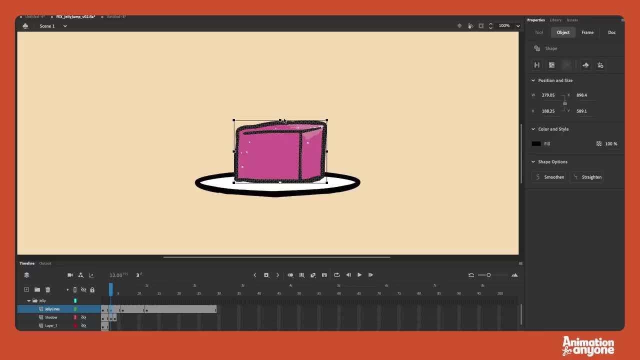 but in this example I'm not going to, I'm just going to transform it. So I'm moving the center transformation, like the orientation point for the transformation, down to the base so that as I transform it the base doesn't move around too much. I'm going to squish it down. 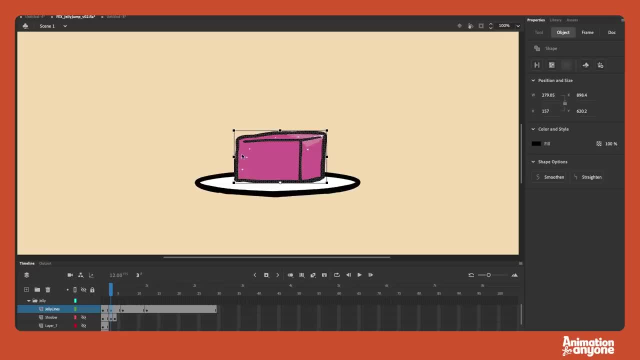 and then what we know about squash and stretch is that it needs to retain volume. So if I squish it down, it also needs to squash outwards and let's just see if that feels about right. I think, yeah, I think maybe just a little bit further out. Yeah, okay, I think that's about right. 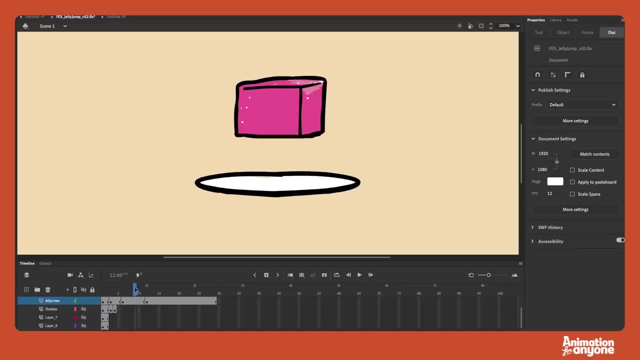 It goes into the air, And then I'm going to have a squash pose when it comes back down, and this squash is a bit of overshoot. So I'm just going to make a new keyframe here. I'm pressing F6 and that means that this one 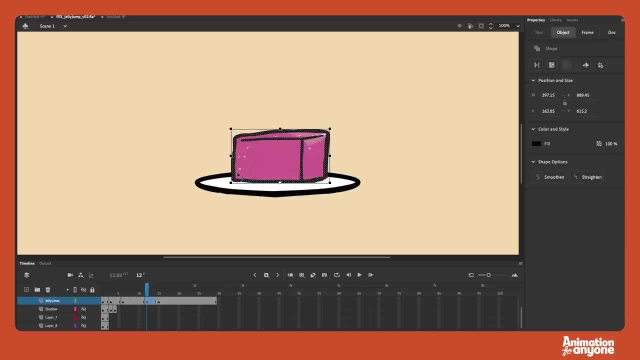 I can squash down, do a similar thing to what I did with anticipation. So now I have the extremes. So we've got first pose anticipation, we've got the jumping pose, the overshoot and then the settle pose, Okay. so that's pretty cool. Now I think we need to look at the spacing here. So we want the motion to 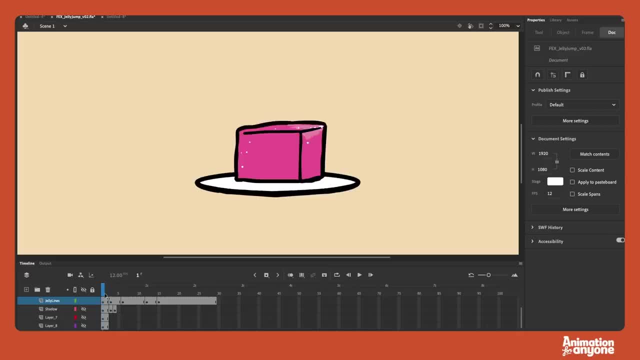 explode upwards, hang in the air and then come back down quickly. So to do that, I'm just going to make a new keyframe. I'm going to make this one ease into this pose that's ahead of it, And then I'm going to ease out of this pose here And this. this is really weighted towards that top. 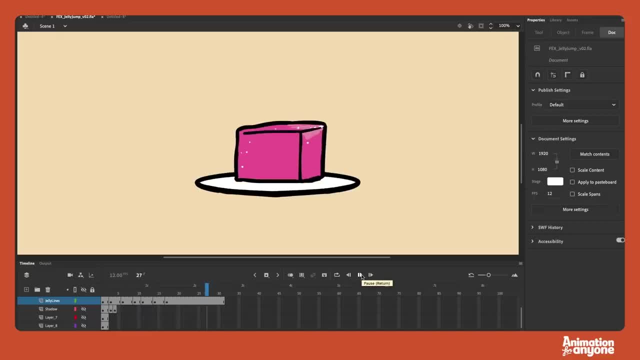 pose. So I'm just experimenting with the pay, with the timing here, And, if I'm honest, I think the timing all feels a bit crazy. So it feels a bit slow in the air, doesn't it? So what I think we need to do is change it so it's not on trees there and on trees, And then I think this overshoot is a. 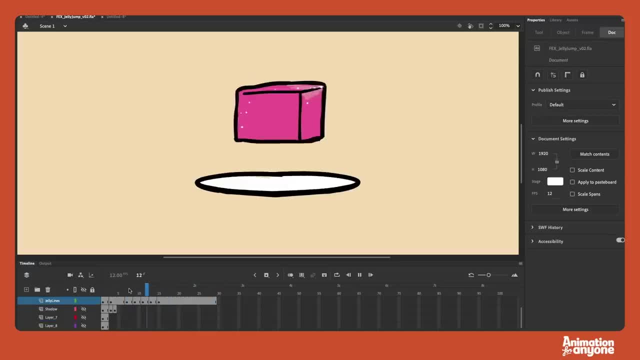 little bit slow as well. So I'm going to move this around. So that feels pretty cool, But it doesn't feel a lot like jelly, And one of the reasons jelly feels the way it does is because it has loads and loads of overshoots. So 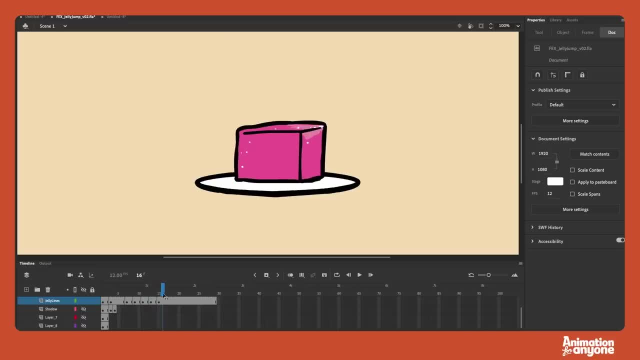 when it comes back down, I think we could overshoot further. So rather than coming to its final pose here, let's just put a series of overshoots that get less and less as they go along. I think that that's feeling a lot more bouncy and fun. At the moment, this feels a bit choppy. 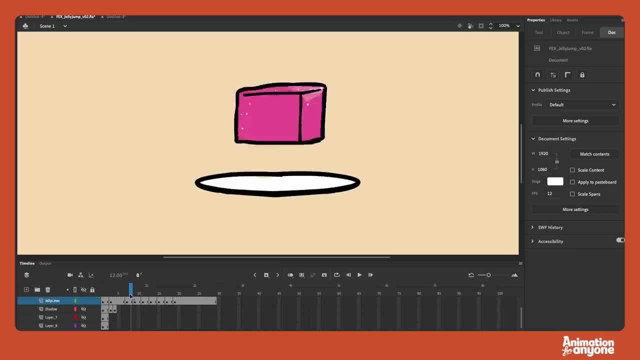 Because the project's at 12 frames per second And we're skipping every other frame, So it'd be good to fill in the gaps with some in between. This is feeling pretty nice Now. There are loads of other things you could try when you're doing it. 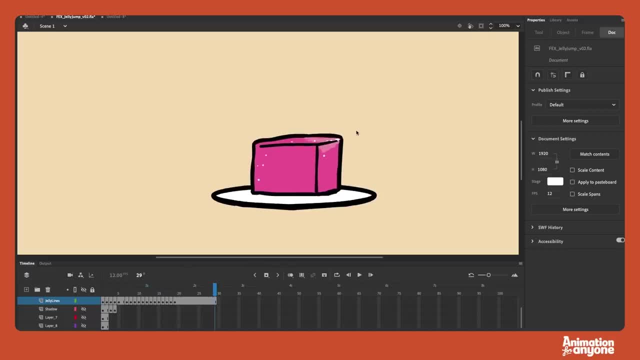 yourself. You could see how many overshoots you could fit in at the end. Or maybe you could play around with adding a stretch frame, like I'm doing here. This is a fun exercise because it's a simple way to practice overshoot And it also makes you think about a pretty common five pose pattern And 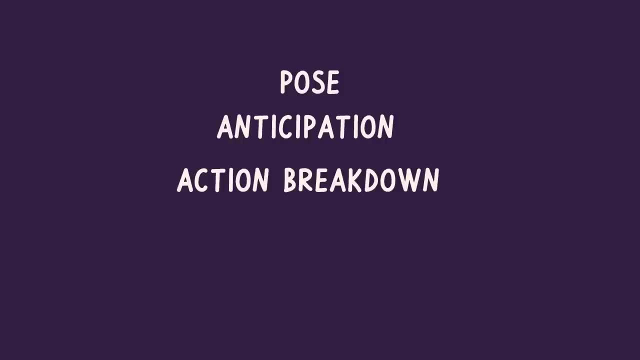 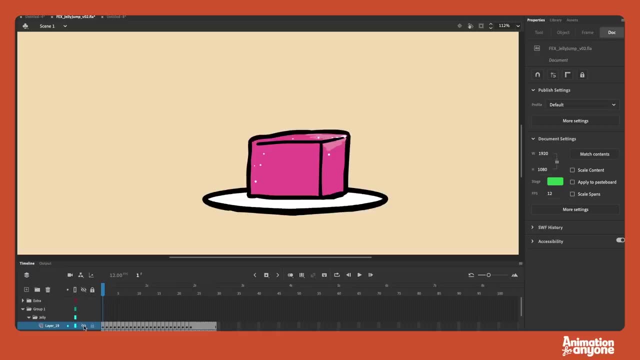 that's pose, anticipation action or breakdown, overshoot and end pose. This is something that's really useful for loads of different kinds of animations, So let's go ahead and get started. If you want to make this exercise more difficult, you can try putting another cube of jelly on top. 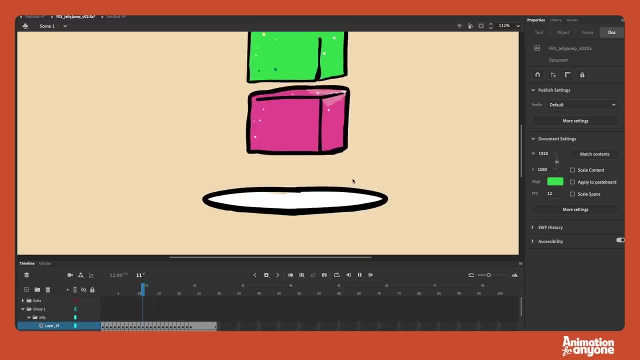 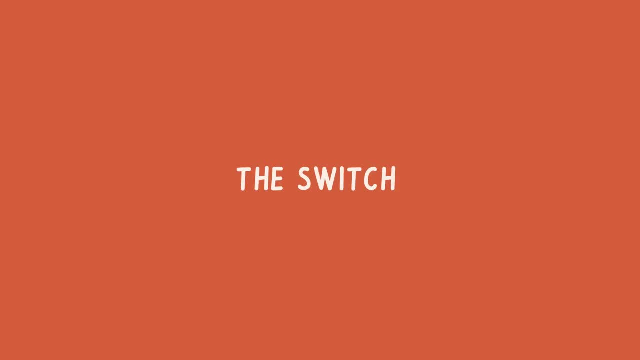 and animating it responding to the cube below. This can get tricky as you start to think about how all the shapes are interacting. A third exercise is something I call the switch. Our goal here is to transition between two very different keyframes as quickly and easily as 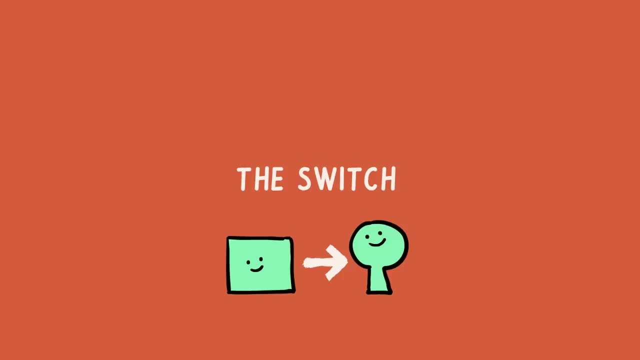 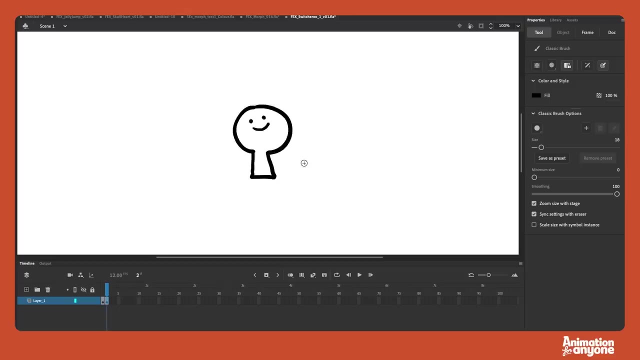 possible. We'll do this by hiding the transition behind motion. This is something that sleight of hand magicians use to hide things from the audience. This is something that you can do in animation. You could take a lot of drawings or some sort of real sort of thinky problem solving. 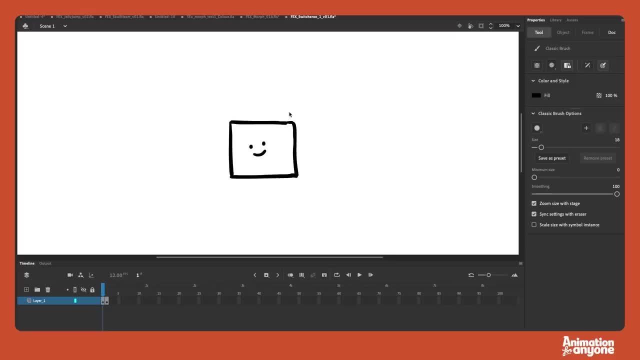 to figure out how to get from this keyframe to this keyframe, But what I want to do now is show you that you can hide this morphing behind some motion, and your audience's brains will fill in the gaps for you. I'm going to duplicate this keyframe And because they're basically at the 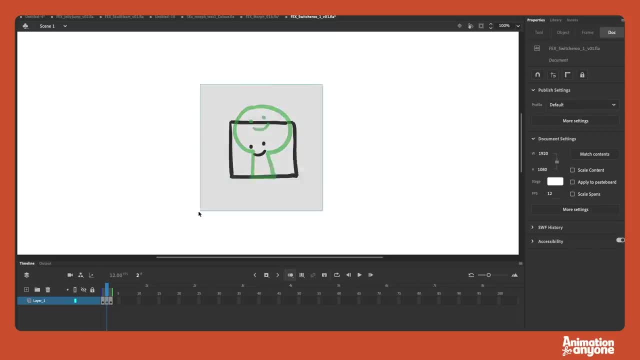 same spot. I'm going to use anticipation like a little jumping motion And then I'm going to duplicate this keyframe to hide this transformation. So we anticipate down And then for this pose I'm going to duplicate it, I'm just going to overshoot upwards. So this makes it feel like 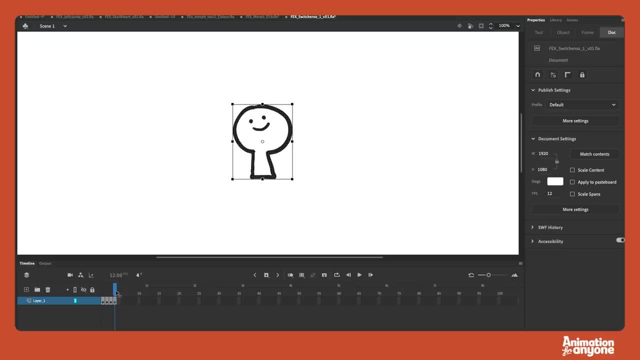 we go down, we travel upwards really quickly and then settle back down. Now we'll just time this out a little bit better. So I'll hold for five frames, anticipate for two frames, overshoot for two and then hold. Now these are guesstimates, So let's see how they work. 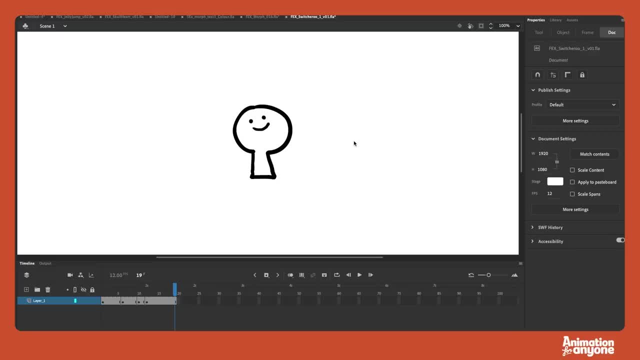 So you can see straight away just a couple of drawings. no real sort of morphing. we're able to get from one keyframe to the other really quickly. And now I'll just go in and fill in a couple of easing. easing in between some, some slow in, slow out sort of thing. 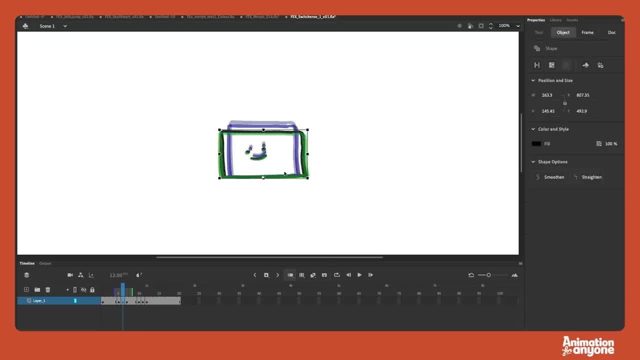 So I'm just going to duplicate this. Let's see how that looks. So you can see really quickly I'm able to get between two very different keyframes very quickly. but we don't always need to use this anticipate overshoot formula if we're moving a. 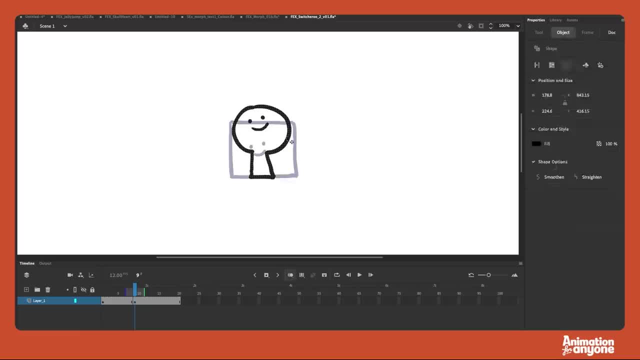 character or object across the screen. So over here we can just use a little bit of easing to hide this transformation. So in this case I'm going to have a really subtle Start to the motion. What this will do is sort of leave a little bit of grace in the motion, and then I'm 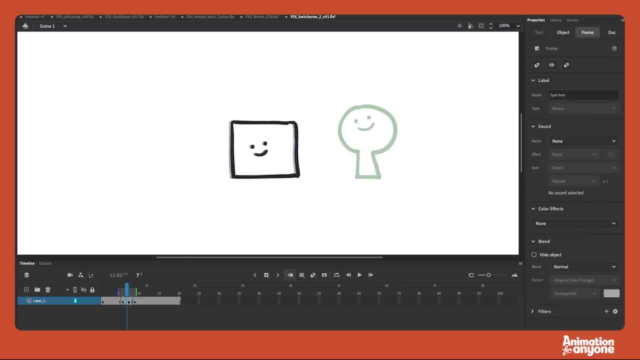 going to move the hemline a little bit further back to the screen. Now we can go back to the moment to see if we could get a little bit of easing to the performative shape of those too. the audience to expect a big movement, and then I'll just keep going across. so 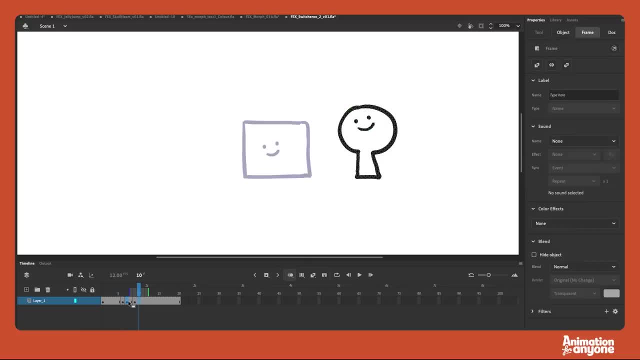 we're building up a little bit of momentum here. now I'll take my next frame. I'm switching right at the, the fastest point of the motion. so so if we switch at the fastest point in the motion, that's when it's going to be the least obvious that we're changing shape entirely. 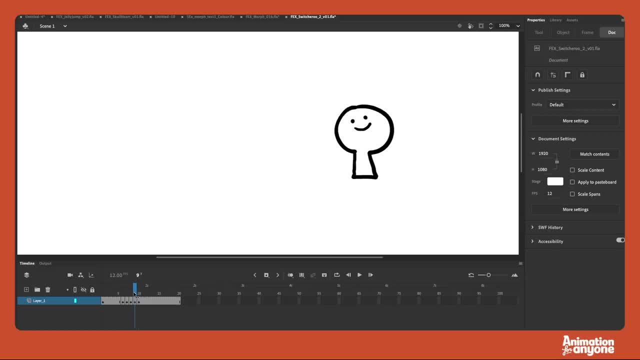 so that works pretty well and I might just make a little bit of a subtle transformation here. it's not essential, I don't think, because most of the works done for us already, but I'm just gonna squash it down a little bit and then I might overshoot upwards here, and that, just you know, relates to the height. 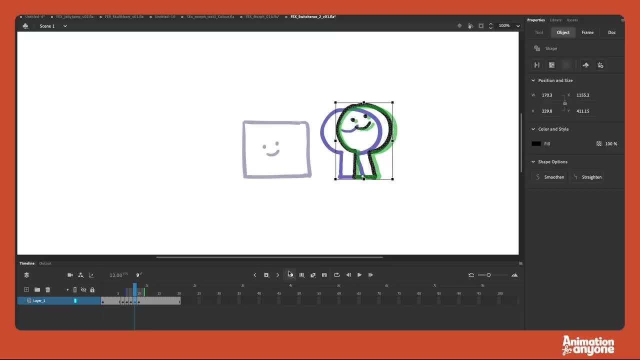 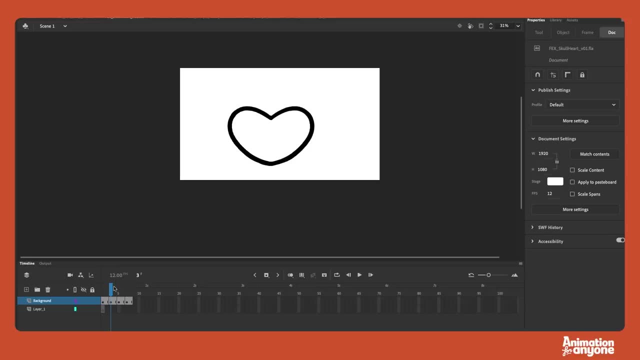 change that's happening. so it feels like it's moving upwards, overshooting and then settling back down, and we can do this. we can use this technique in loads of different situations. so if I want to switch from a more complicated shape like this heart to a skull, you can see I've mapped out a few keyframes here. we've got the first. 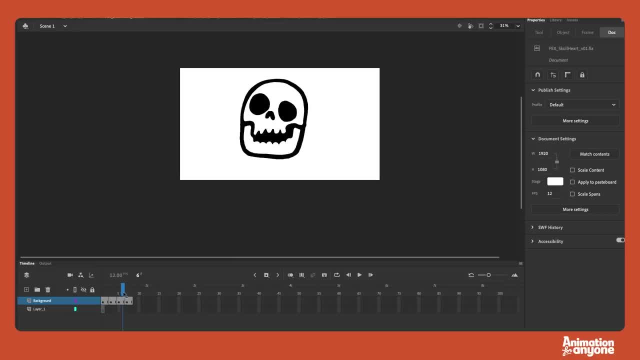 keyframe, the anticipation frame, the overshoot frame and the settle frame. one thing that's different with this example is that I've actually gone to the effort of redrawing these, these keyframes. so this isn't just a transformation of the other keyframes, but it's a transformation of the other keyframes. so this isn't just a transformation of the other keyframes, so this isn't just a transformation of the other. 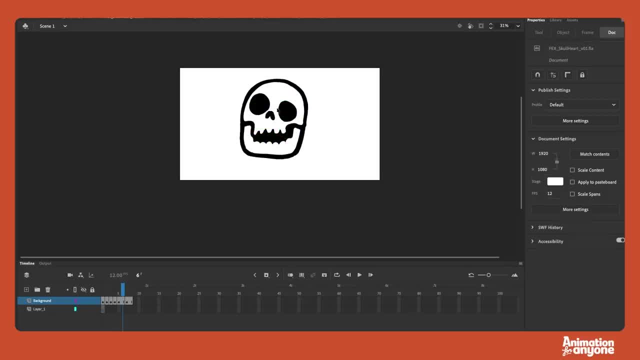 heart frame. so you can see, here I've created stretch in the skull by extending the jawbone down and then it compresses here. so what I'm doing now is just creating a little bit of follow-through, overlapping motion, so that it feels like the jawbone follows the skull up a little bit. that just. 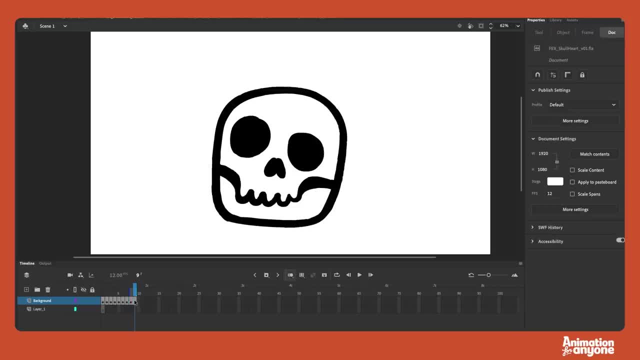 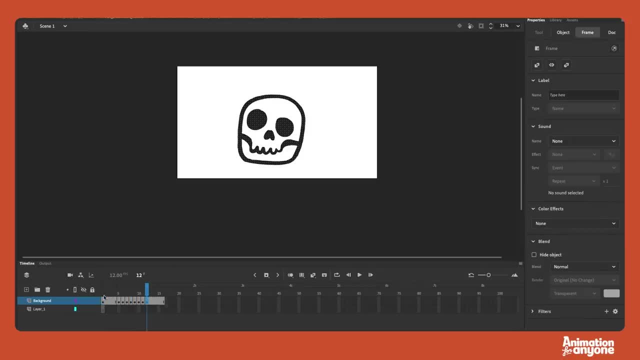 loosens things up a little bit. now I'm just gonna overshoot a little bit with the skull just to give it a bit more weight. I'll test it out, maybe retime it a little bit now, so you can see straight away that this would have been quite a hard thing to. 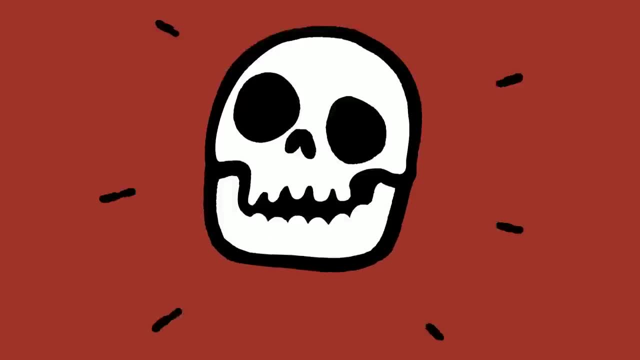 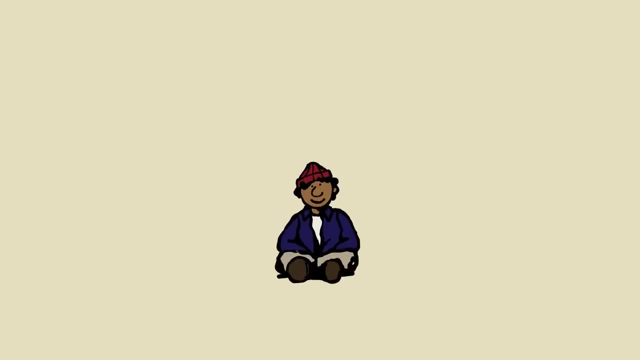 morph between, between this thing and this thing. they quite complicated shapes, especially the skull. if you want to really push this idea, you can even use it to create stylized character animation by popping between key poses. a fourth exercise is called the morph. this is a lot like the switch, but rather 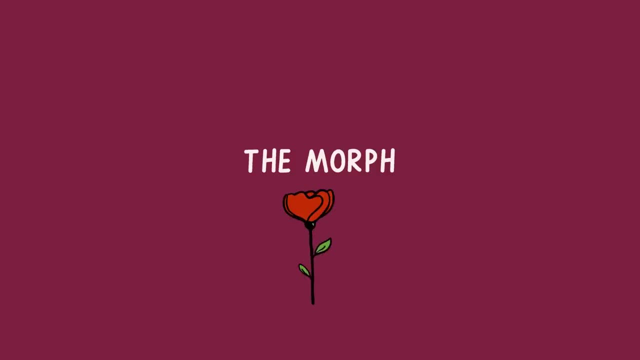 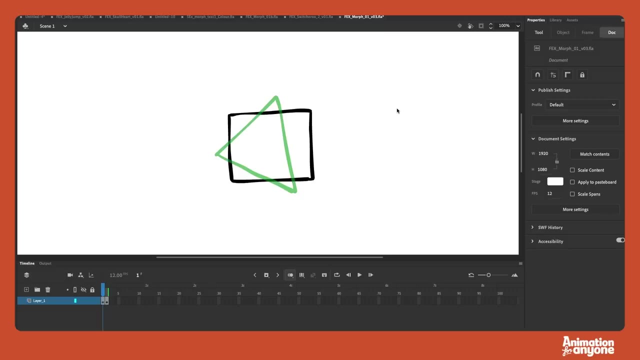 than hiding the transition between two different keyframes, we're going to exaggerate it. so with this exercise, we want to take two very different keyframes and blend between them. in this example, I'm using a square and a triangle. the simplest way to do this would be to overlay the two.